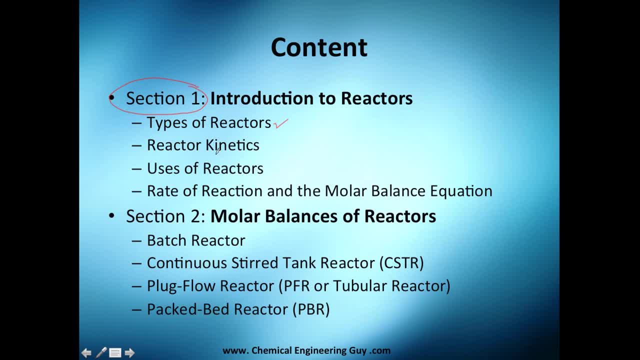 introduction to reactors. what type of reactors do we have? some reactor kinetics and the uses of those reactors. Then we're going to see a lot of pictures. I'm going to try to explain you how to recognize or to know what's a reactor in the chemical industry, And in the second video we're 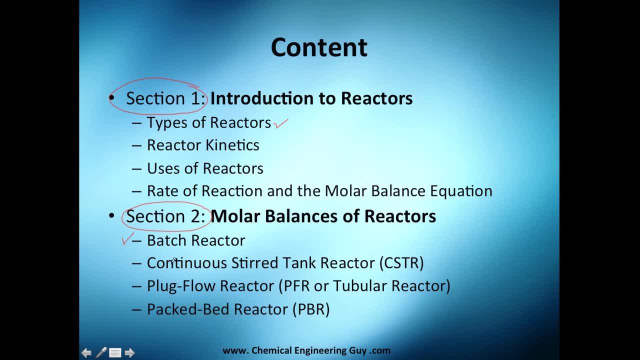 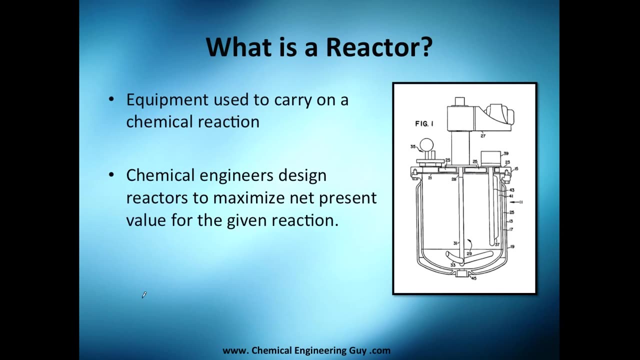 going to jump to molar balances, which are done essentially in batch reactor, continuous-tier tank reactor, plug flow reactor and packed bed reactor. Right now we're going to see just the introduction to reactors. So the first thing I want to let you 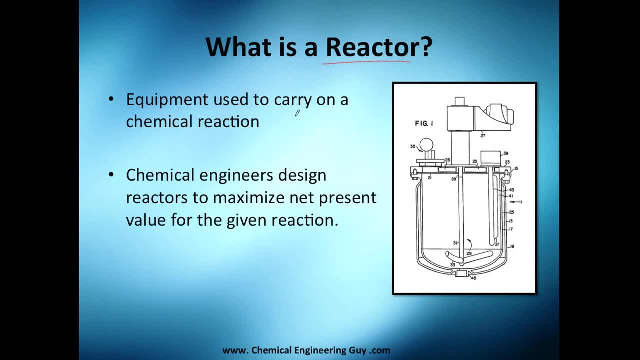 know is: what's a reactor? A reactor is? I tried to look out for many, many definitions, but I think the most common sense definition is this one: It's an equipment used to carry on a chemical reaction. So, essentially, if you have a mixing unit and you're not doing a chemical reaction, 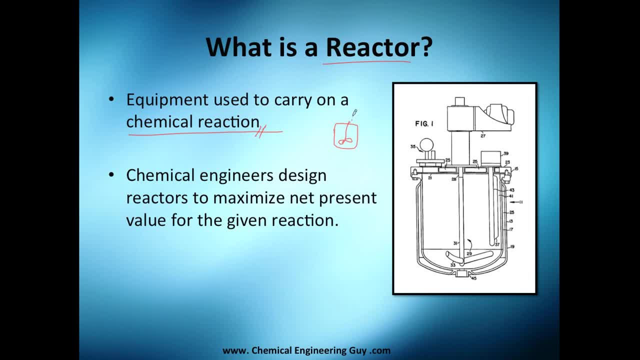 that's not a reactor. But if you are carrying on- I don't know- A turns into B, then you are doing a chemical reaction. Therefore that's a reactor, And actually there's also types of pipes You're using. 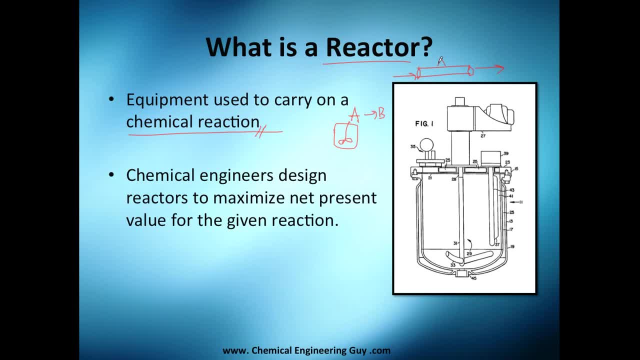 this pipe just to transport material and, you don't know, you're transforming A to B. Technically speaking, this is a reactor. Of course we don't want to do that. We want this pipe to transport A into, of course, only A. 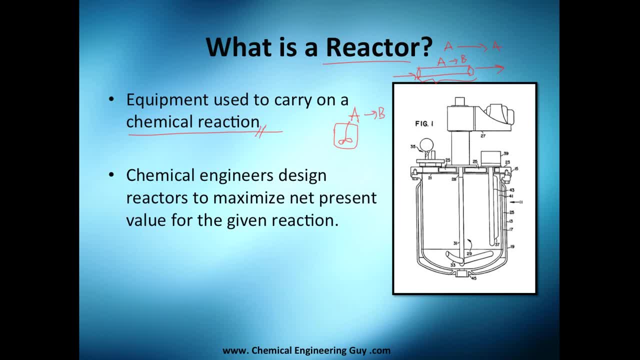 transformations. but technically speaking, if you have something, a device or equipment that transforms a chemical reaction, then you have a reactor. so yes, chemical engineers design reactors to maximize net present value for the given reaction. so that's kind of fancy. what does that mean? is essentially: you want 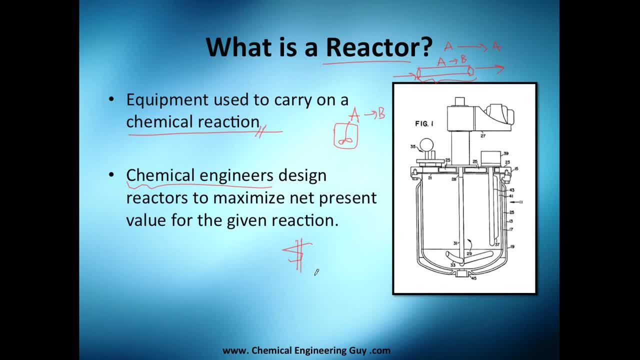 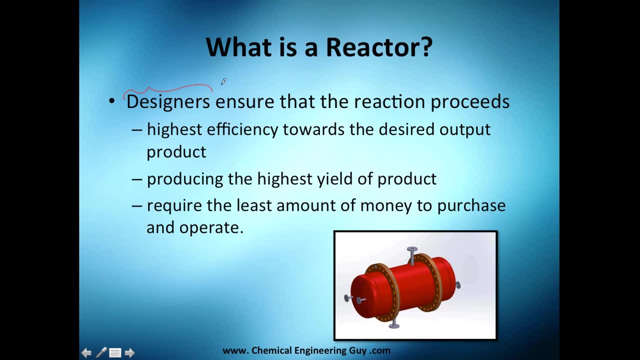 to improve the reaction in order to get more profit. so let's keep doing. how do we do that? the designers- which looks like a fashion design, but now it's not fashion, it's a engineering design or reactor design- ensure that they got the highest efficiency possible. that was the desired product. so you're turning a into. 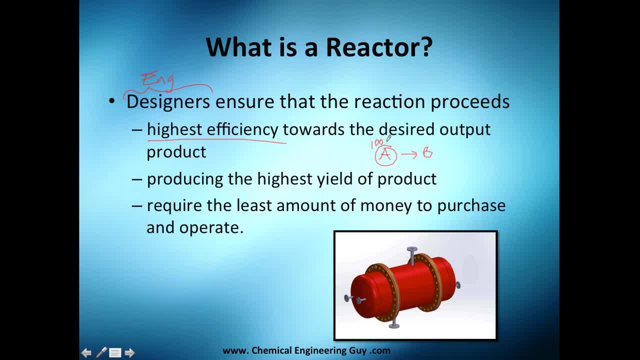 B. of course you want to turn all a into B. sometimes you're not going to be to be able to do that, so you're going to find out or design a reactor or try to change temperature, pressures, flows, whatever you need to do to prove that conversion rate, and actually you're going to base all these in money. so of 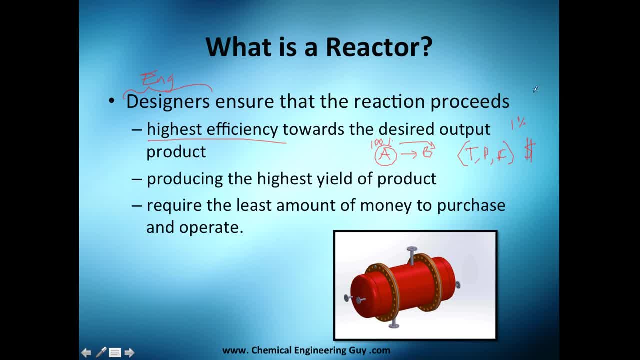 course, if I tell you I'm going to increase one percent yield but you're going to need to invest 1 million dollars, well, you need to check out if it's actually worth that one percent. so yeah, that's the highest yield of product and, as I told you before, you need to require the least amount of money to 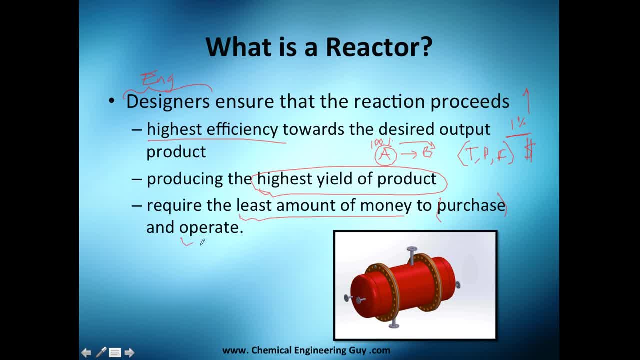 first of all purchase, or to invest and to operate, because one thing is having the reactor, the other thing is actually operating. you will need someone there taking care, someone that cleans, someone that operates control, temperature, heating, cooling, piping, pumping, compression, all those stuff that are behind the operation. 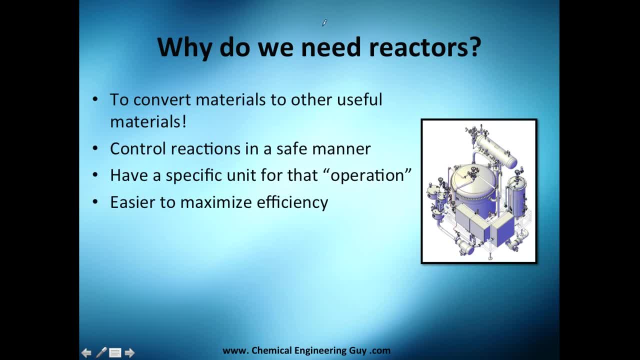 so why do we need reactors? well, we want to convert material. that's what I love, chemical engineering. it's about transforming, converting, producing materials which are not that useful or which maybe they are useful but you want to turn them into something else. so let's say, you have these low value. 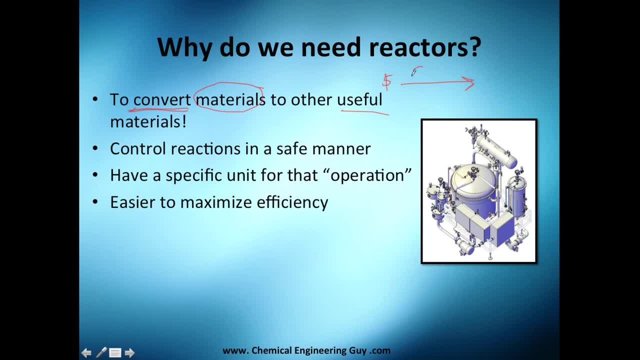 material, and I love it because you use your knowledge, your brain, and you transform it to more profitable materials. so that's why I love chemical engineering. let's do some magic with our knowledge and we get more money with that. we do it because we want to have a specific unit for that operation, so at least we know that this. 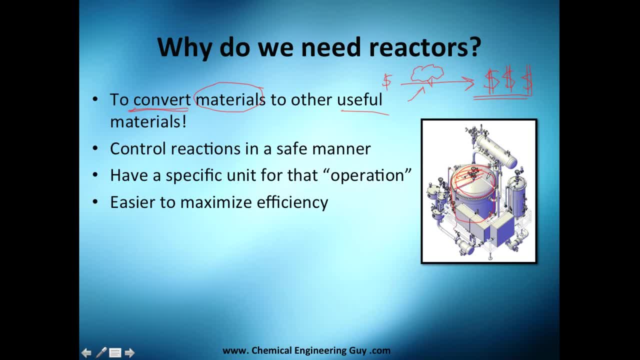 tank is where our chemical reaction is taking place. so if you don't have in the- let's imagine- this plant or chemical plant, you have a problem. you're not getting the yield or the conversion you want. you go to the reactor, you study the reactor here. you don't need to check this out or this out or this piping here. 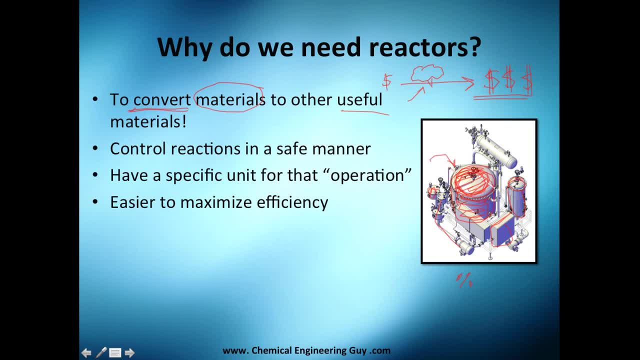 maybe eventually you find out that the reactor is fine. you will need to do that, but the first thing you want to do is to go directly to the reactor. so that's why we are doing this in one reactor and not in many operation units. so essentially, you want a specific point or space. 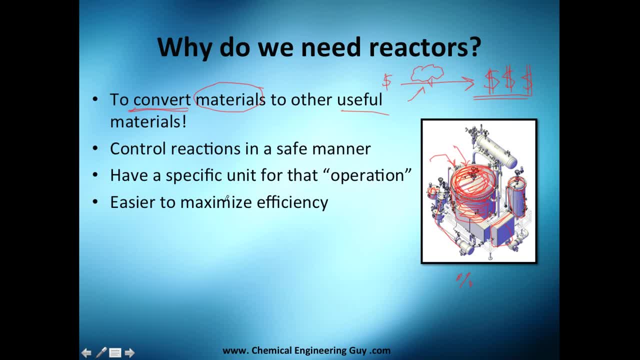 where the reaction is being carried. and not only that, you also want the reactor to control the reaction in a safe manner. so you don't even know where your reaction is taking place. well, that's not that safe. you know you're taking place in this tank. well, at least you're going to make that tank the most safe place in. 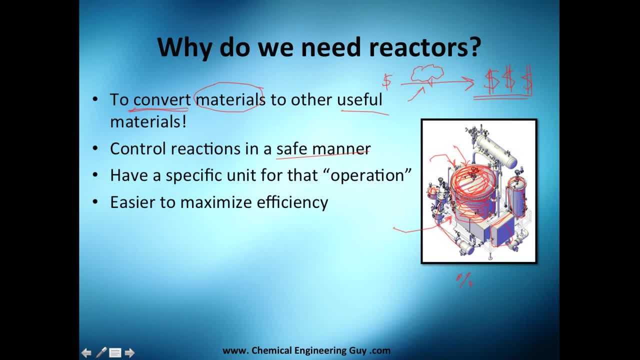 the plant, or at least that it doesn't explode or leak or whatever stuff or thing may happen that may be hazardous for health or environment or workers, whatever. and the thing here is that it's easy to maximize efficiency. why? because then you're going to work fully on this reactor and not in the whole plant. so 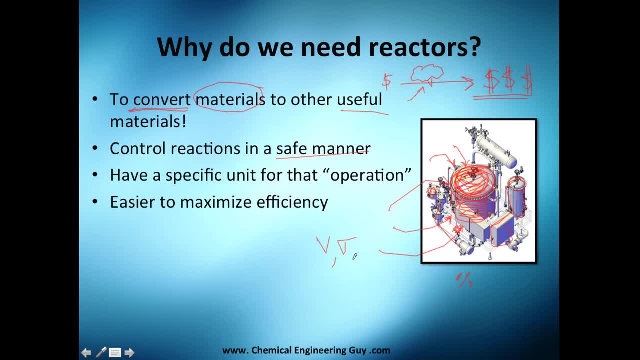 you can- I don't know- change the volume, change temperature of flows, pressure of flows, concentration, all those process variables that affect the conversion rate or yield. you can change them. so that's kind of cool, because you're going to change also levels, temperatures, inlet, all those things that you can change you're going. 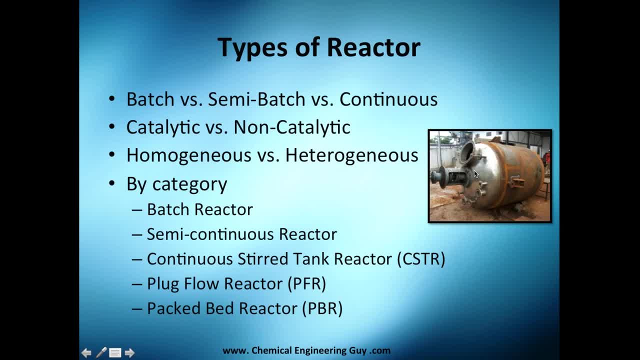 to do them in this specific unit. so the next thing we're going to see is the types of reactors. there are many, let's say, types of reactor or how to order them or classify them, so I brought you the most common and the ones you're going to be using, for example, batch. or you can say also: is that semi batch? 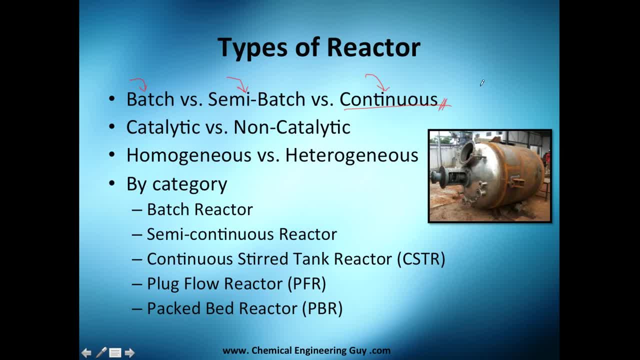 process or a continuous process. this is in general. you have a plant operating all the day, all the year long. you transform A to B, let's say in this reactor, and you have a flow of temperature 10 kilograms per hour here and you take out 10 kilograms per hour of B. this is A. 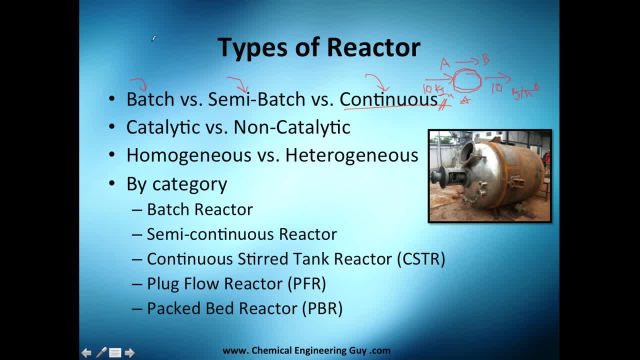 it's an example. a batch is essentially just: you got this tank, you feel it up, you let time pass, it reacts and you take it out. a semi batch is a mixture between a batch and a continuous. that's one form. another type of reactor. classification is either is it catalytic or not. 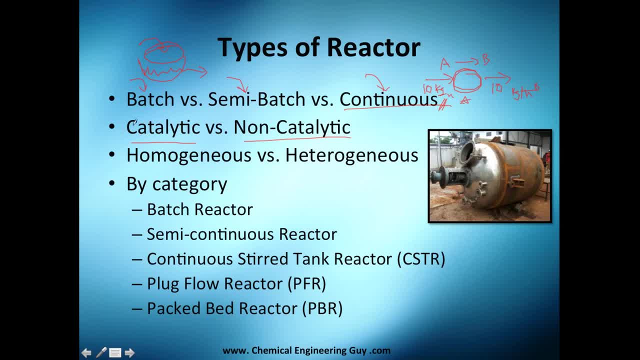 catalytic. when it's catalytic, Catalytic, of course, as the name implies- you have a catalyst, and when you do not have it, well, it's a non-catalytic reaction. Then homogeneous reactor, which means there are the same phases, let's say liquid-liquid or solids-with-solids. 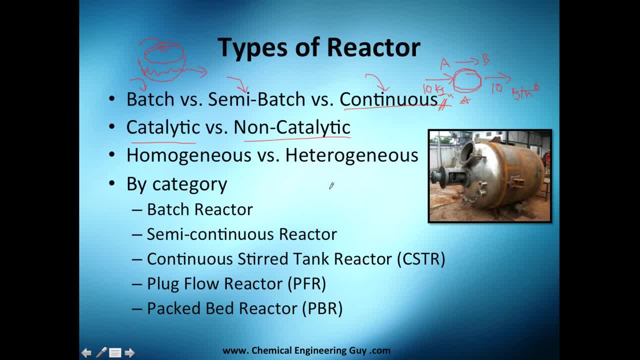 and then you have the heterogeneous phase. for example, you have a gas here and this is like a packaging. you need this solid, so they react or they do a process here and they interact between solid and gas, which is a heterogeneous reaction, and you take out this here, so that's also important. 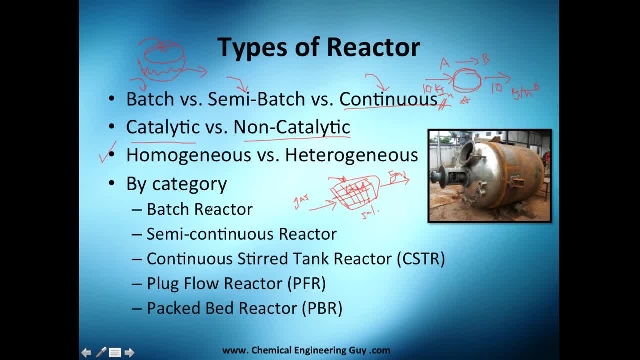 And the most, I think, the most important thing to know is these categories, which is the reactors we're going to be studying in this course, this introduction to engineering, chemical engineering reactors. So the batch reactor is the most classic and obvious one. then comes the semi-continuous reactor. 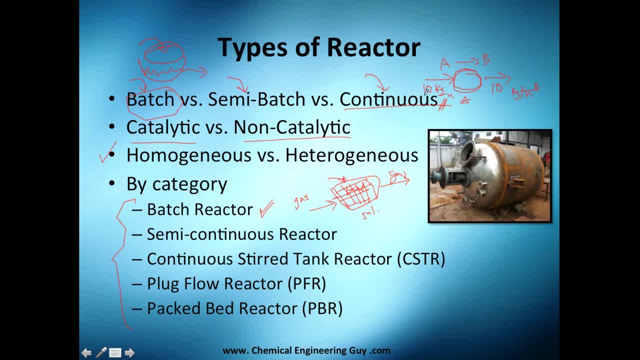 which I told you is a part batch and part continuous. Then we go to a continuous-steer tank reactor, which is the most, I think, basic and easy to model one. You have a tank and, as the name says, it's continuous. so you have this flow and this flow. 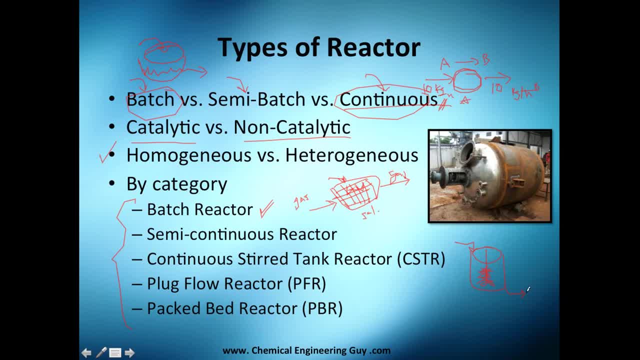 and you mix, mix, mix And react and take out the product. So, as you can see, it's a tank which is steered continuously and it makes reactions. Then comes the plug-flow reactor, which is essentially some pipelines here. 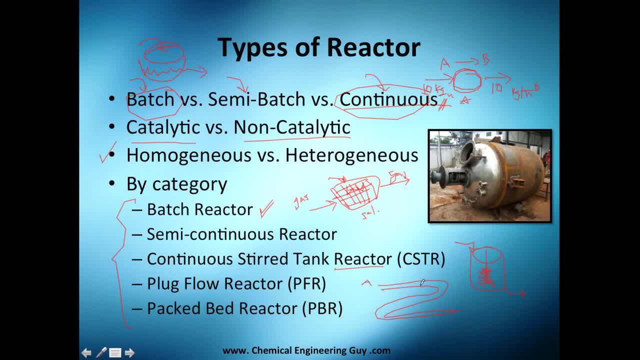 You are reacting the material in the pipes. so you got A and it start reacting all over here and you get out B, And then the packed-bed reactor, which I told you. this little example: you have this reactor, you got this packed-bed here. 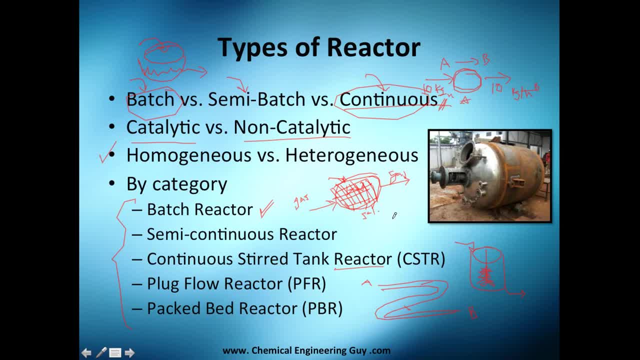 And you are reacting I don't know gas with this solid and you take out the product. So those are the type of reactors. please, This is kind of theoretical. I know it because I've done too much of that. I actually didn't like memorize it. 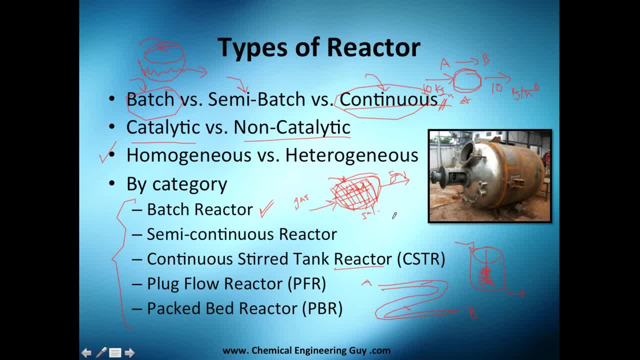 You don't need to memorize it. You're going to be working with them and you're going to see the characteristic of each of them. For example, continuous are in steady state. Heterogeneous normally implies a packed-bed here Batch reactor. 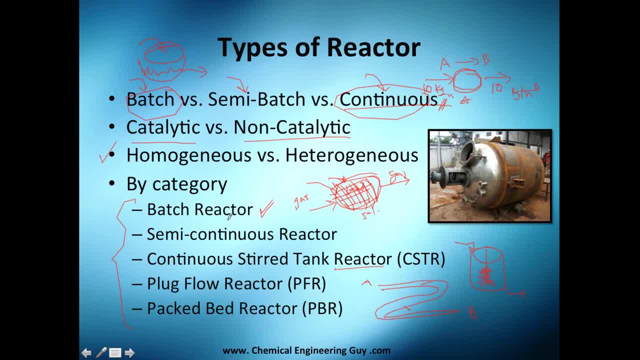 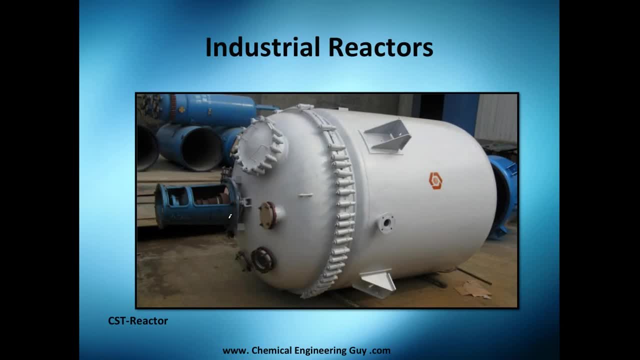 It means that they are time-dependent And with the time you're going to recognize each of these concepts. And now I brought you some pictures. I want you to realize what's a reactor. Look at this tank. You can see this is like the over part and this will be the whole tank. 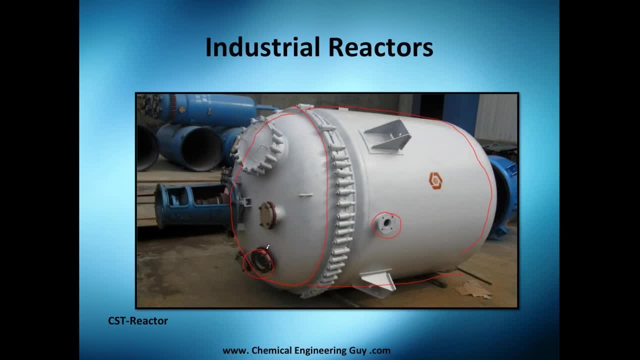 This is an inlet, maybe, And this outlet here, or maybe this is the inlet and this is a level, Then you've got this part here, which is where the agitation unit goes. So you have this unit here. It goes all the way down. 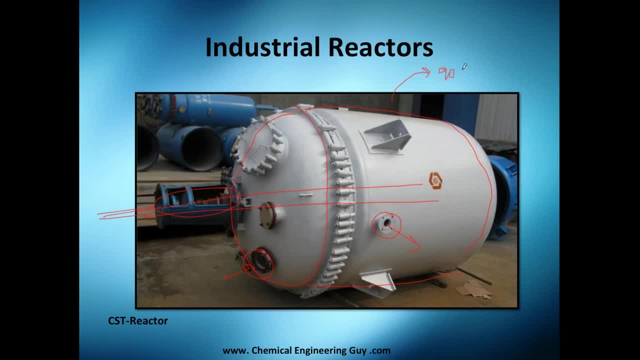 Of course, this should be 90 degrees. This is, let's say, laying down. So you need to stand this tank up and you will have your agitation unit here And you're going to mix it And this, as you can see, is a tank. 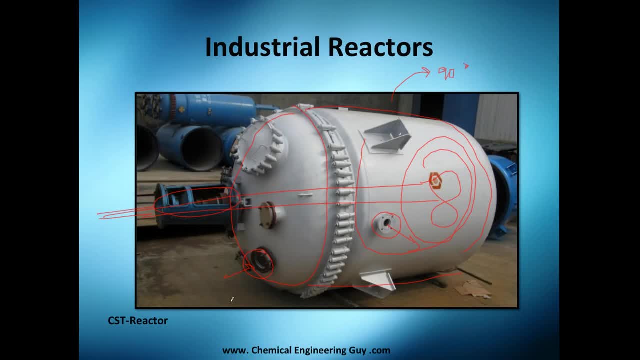 And you have this steering system here. So, as you can see, it's a continuous-steer tank reactor, because you have the inlet here and maybe an outlet. I don't see the outlet, but it should be there, And this is the manhole. 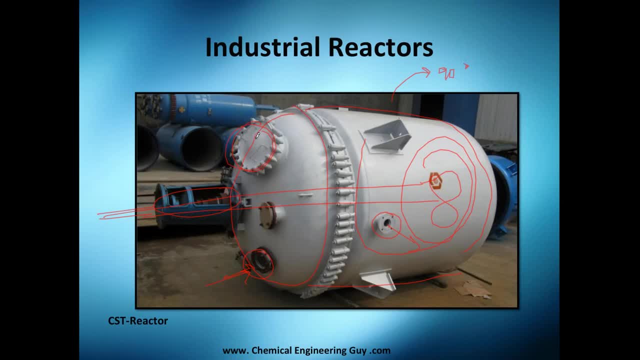 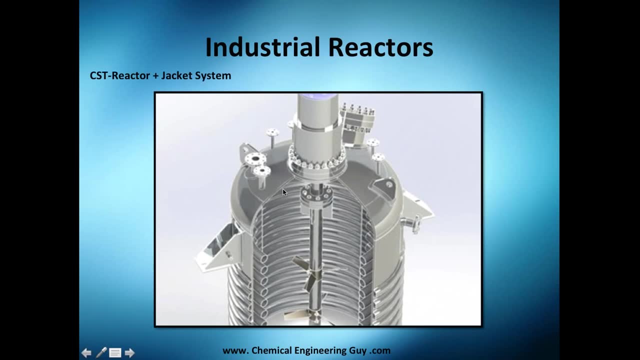 What's a manhole? It's essentially a place in which a man can go in and you clean it or you can check if there's something stuck, or something like that. Then we have still a CSTR or a continuous-steer tank reactor. 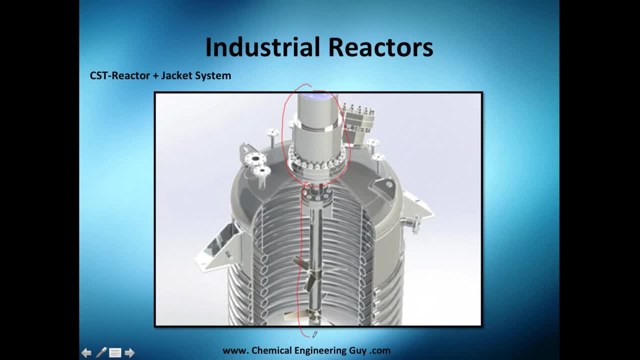 You can see here, It's the thing we were talking about. This is the steering unit, But we got this now a jacket system. What's a jacket system? We're going to see that later, But essentially it's just a lot of tubes that are heating this reactor. 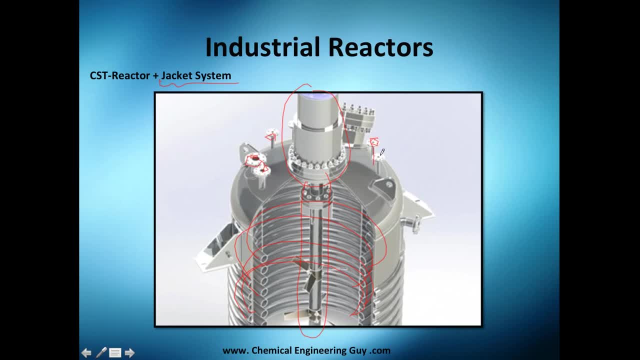 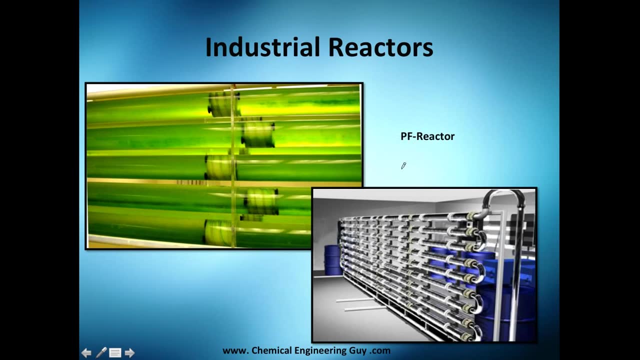 You can see you have many inlets here made for levels, temperature sensors and the manhole. Now we are in a plug-flow reactor. As I told you before, it's essentially just pipelines. They go here and go here And as they move they are reactors. 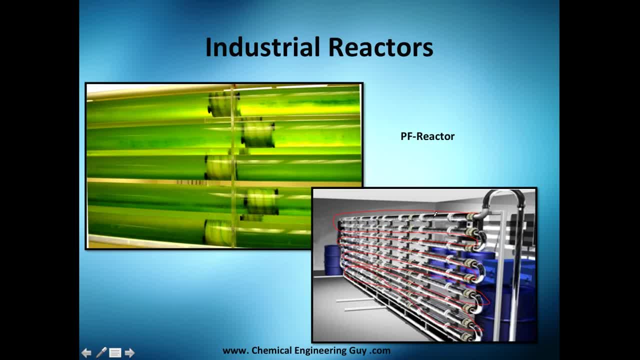 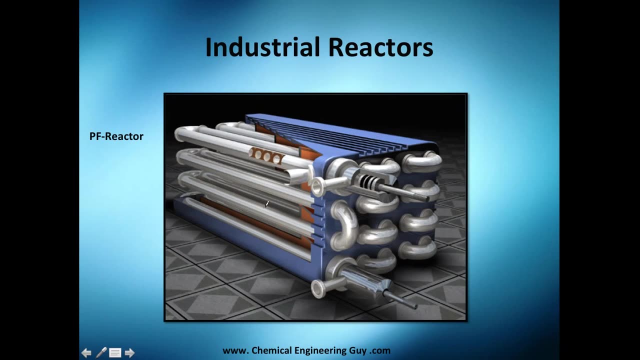 They are reacting the materials. So eventually, if you were having A plus B here and your reaction is something like this: you're taking out C, out here, The same here. Now we have a different arrangement And you actually cover this, so maybe it's more like aesthetic. 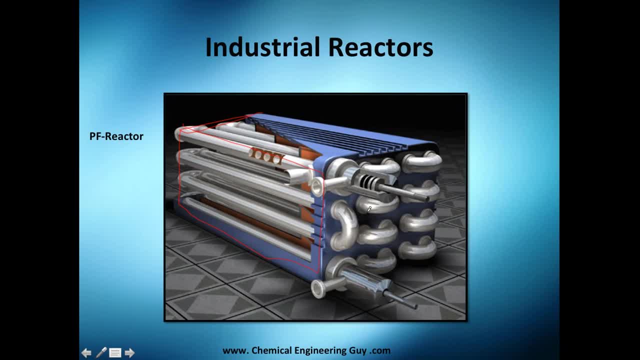 Maybe you're selling the reactors. You want to do it as aesthetic as possible. But actually in the chemical industry you're not looking that into aesthetics. You are more into usefulness, efficiency and that. And it makes sense, because if I were an engineer I wouldn't care. 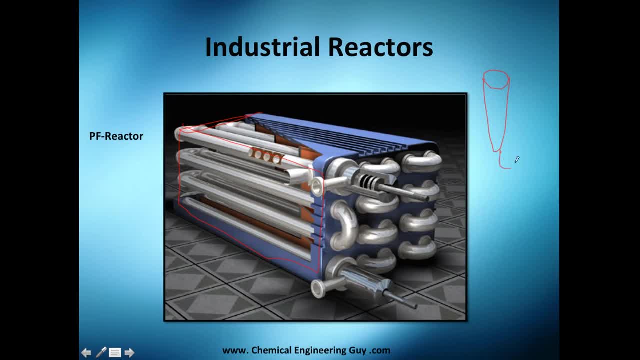 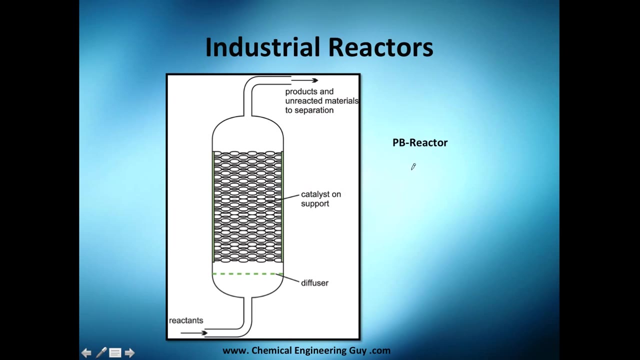 It is not fashion at all. But if it works it turns my material A into B And I can sell B way much expensive. I will not care about the fashion elements. And then we have a packed bed reactor. It's essentially the same tank. 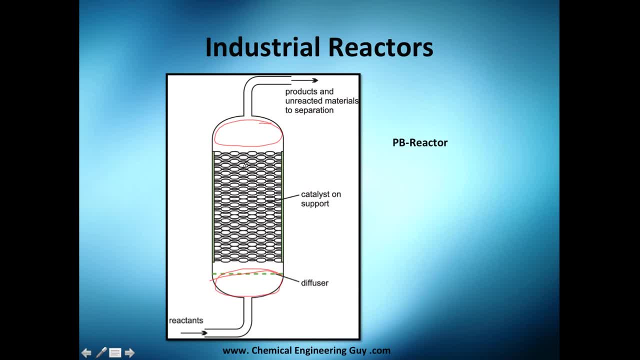 This is the diagram, Because if I give you the photo, you will not be able to see the packaging, of course, Because this will be cover of all metal walls. You have the reactants. You take them here. Maybe this is gas. 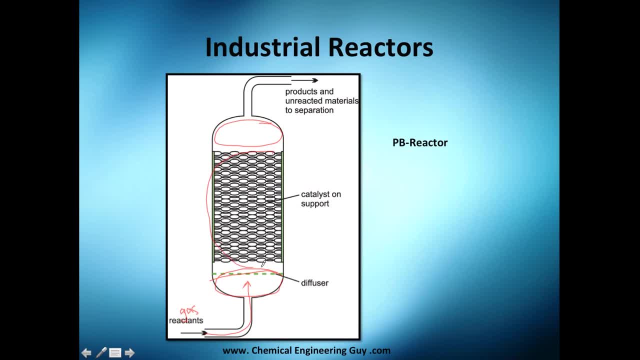 And this is a catalyst. You have the catalyst on this bed or this solid part, So they react, They make their reactions And you take out the products. It's not that difficult or complex as it seems. It's so easy. 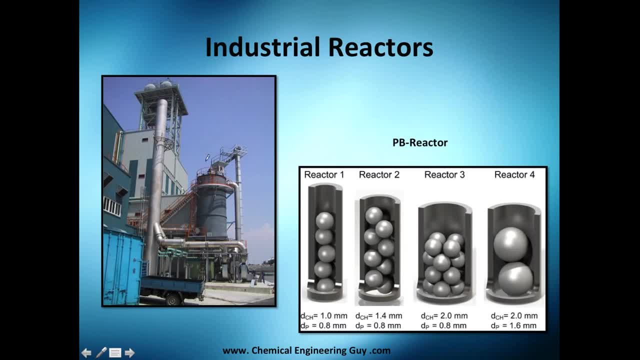 Then, yeah, still, we're talking about packed bed reactors. As I told you before, you can see there's nothing, It's only metal. You can see the packed bed So you could have different arrangements of pellets. Pellets are these balls or these catalysts? 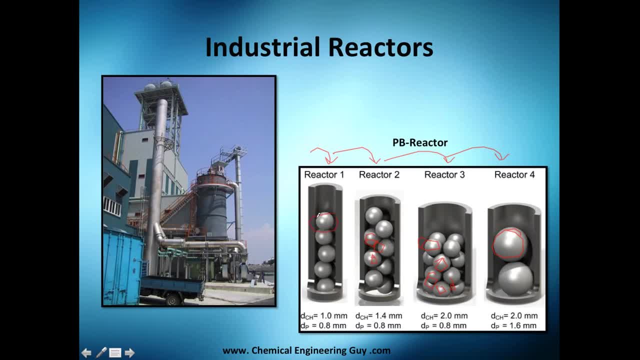 These contain the catalyst, So you could either have a slick or slim here, Or you can have a Wider. You have many small pellets or big pellets, And obviously it depends on what are your requirements on pressure drop. You want to increase conversion. 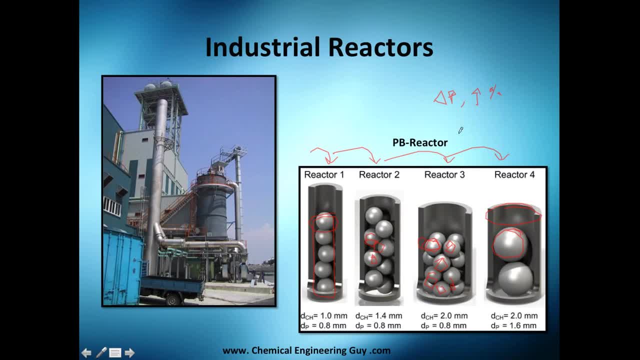 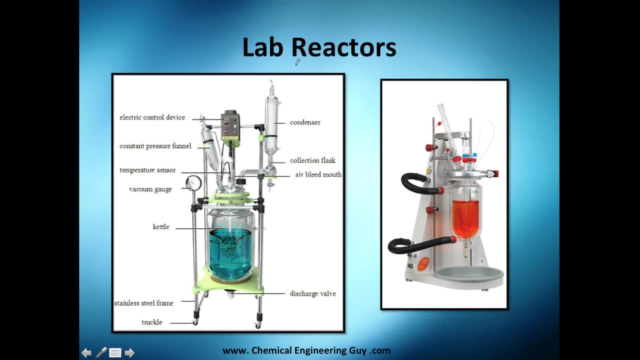 To increase the surface area. There are many, many things that you might want to consider. It's not just about: okay, just pull them up here. So we're now in this subcategory, which are the lab reactors, Or reactors that are done on lab scale. 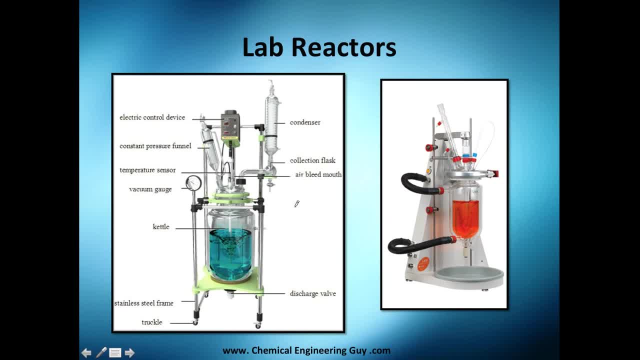 You can see they are simply. You've been in a chemical or a chemistry lab, You can recognize this is like a small beaker. You have all these supports. You've got this little condenser, which has nothing to do with the industrial condenser. 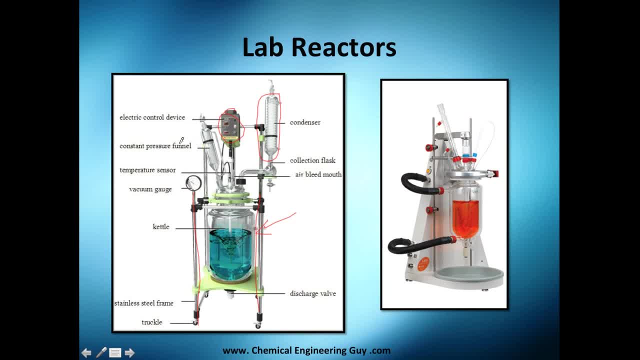 And, yeah, you have all these electric control device, You've got this constant pressure funnel, All these discharge levels. Of course you have an inlet And, as you can see, this is done to improve the reaction. So if you can improve them in the lab, you can improve them, maybe at the larger scale. 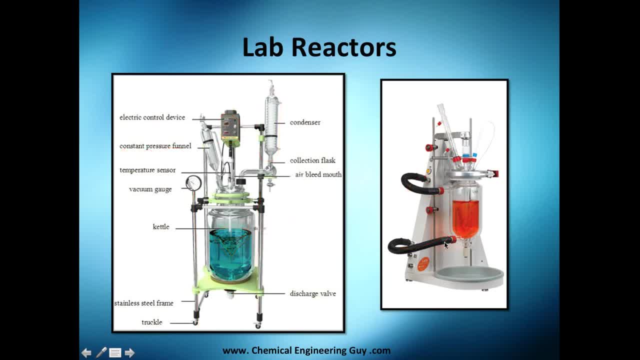 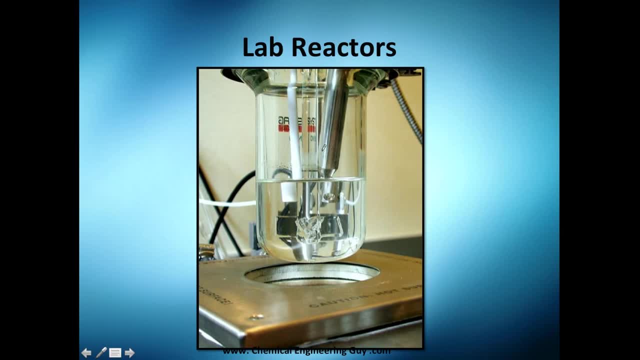 So the same here. Normally you use chemistry workers or chemists or even also chemical engineers to improve the reaction. The thing here is that you want to improve the yield, Or maybe you want to lower a temperature or heat requirements- Viscosity- so you get lower pumping cost. 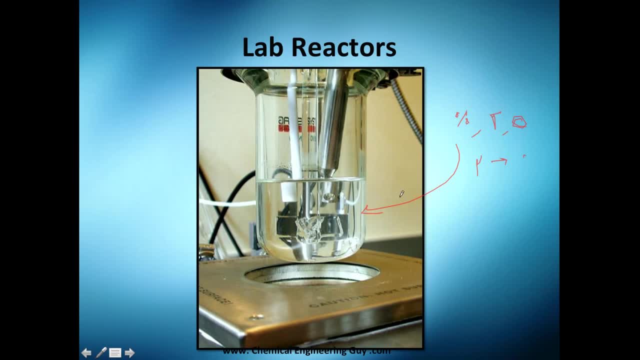 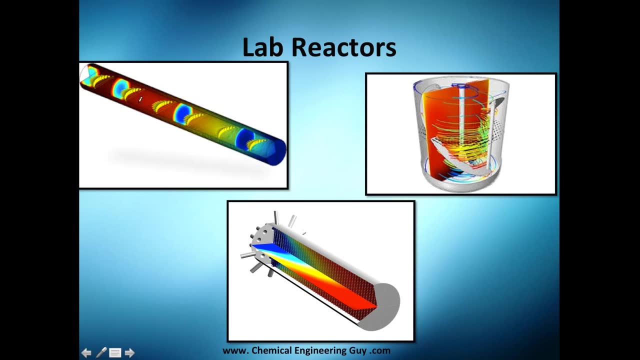 All these things that might interest. you are here And normally you also want to model that, So you can model the lab one or the lab experiment. You can see how I don't know many transfer materials. Maybe this is momentum transport. 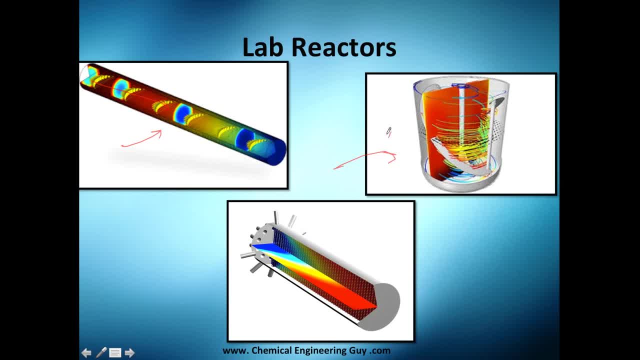 This can be a heat transfer Or not. this Actually, let me just say this- A heat or temperature profiles. These are momentum or velocity profiles. You can see all the agitation here And maybe this is the mass profile: How they're changing this. 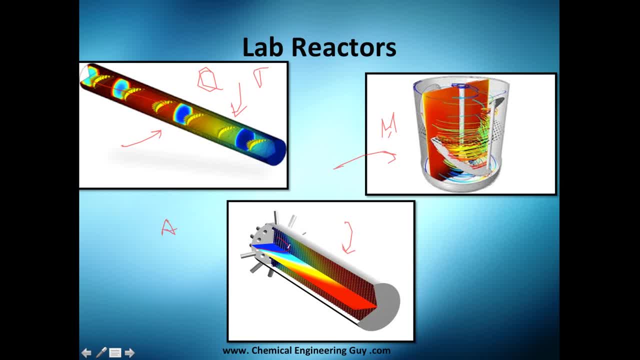 Let's say the blue one is A and the red one is B, And A is turning into B. So you can see how at the beginning you have a lot of A and at the end you have a lot of B, Which makes sense, because you are transforming A into B. 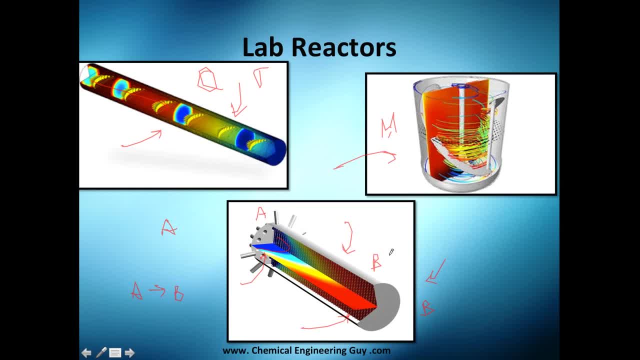 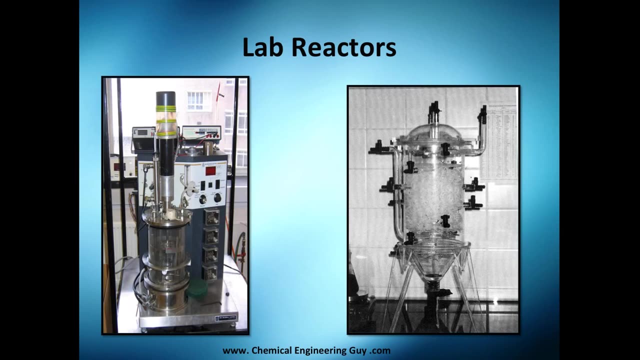 So that's why you can also get some lab reactors. You want to improve and model and eventually just get a better version of your real reactor in the chemical industry. Same thing here. You can recognize them. Maybe this is a CSTR, small scale. 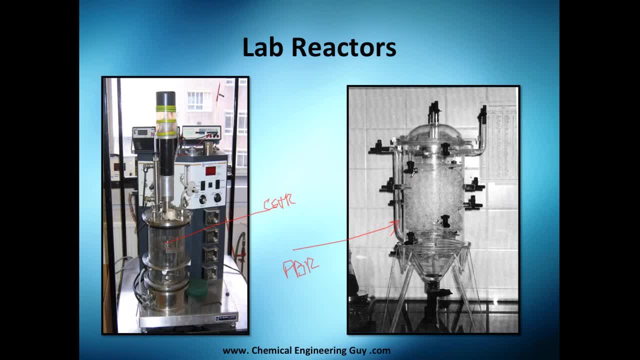 And this is a PBR. of course You have this packed bed. As you can see, you have a lot of pellets, So I am guessing these are A packed bed In which you get here the gas and you take the out. 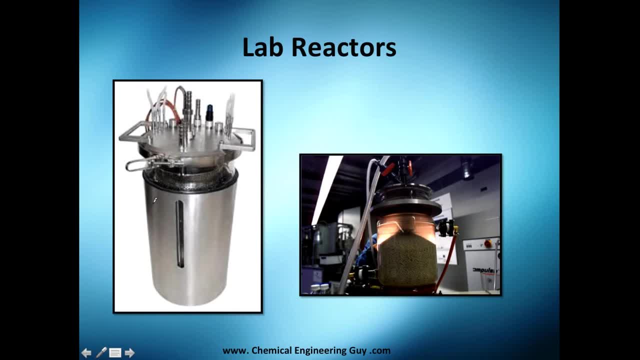 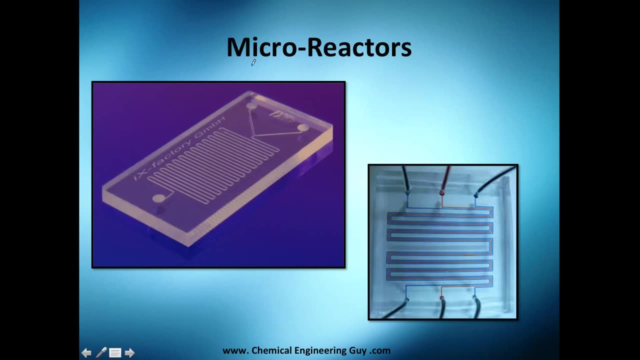 So, yeah, same thing here. Actually, this is also a packed bed reactor, But you cannot see the packaging, Only here. But you need to be watching closely. And yeah, essentially that's lab reactors. We're going to see a new trend, which is micro reactors. 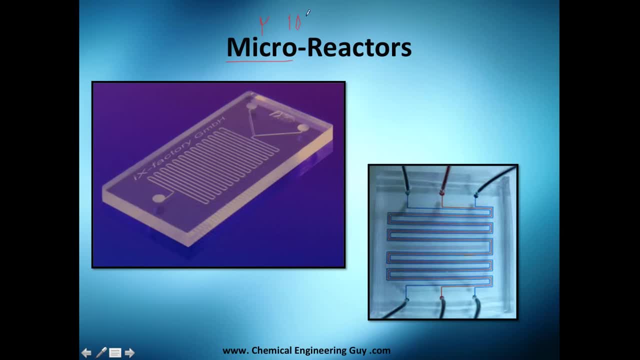 Essentially, as the name says, micro 10 to the minus 6 meters. So Why do we use this? Because we get many At the micro scale. we get many, many good things You can control better. Essentially, it's all about transport phenomena. 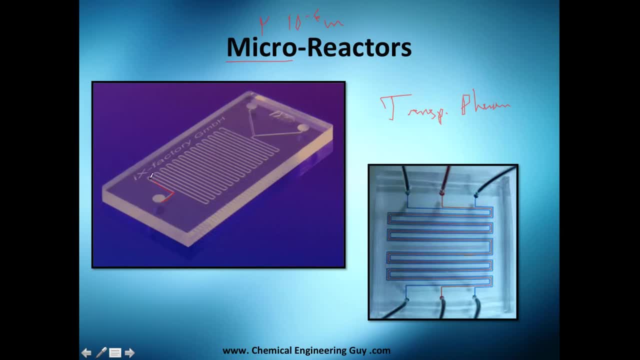 Hopefully you've seen that before Because you're going to get That. you get laminar flow and you get more pressure control And heat controls and all that stuff And Yeah, You can see another here. You get a better control of the reactants. 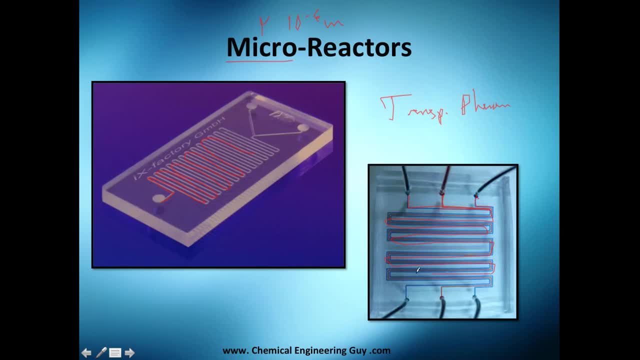 And the thing here is, once you got this micro reactor working as you wish, You can get- I don't know- Maybe 10 to the 6 units, Which is about 1 million, Or maybe you just want 1,000. 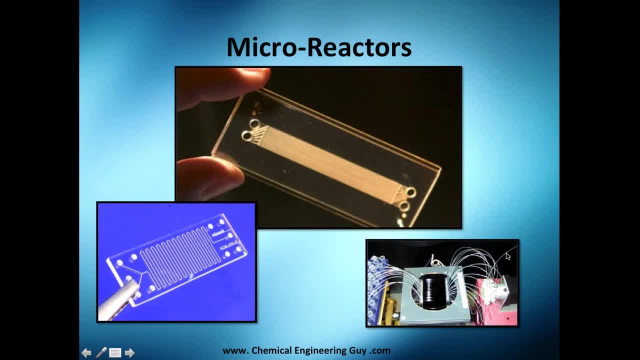 Depending on the flow, of course, And your requirements, But you can get this very scaled up With scaled up abilities. So the same thing here: Instead of using piping, You got these hoses. Small hoses here Instead of getting huge pumps. 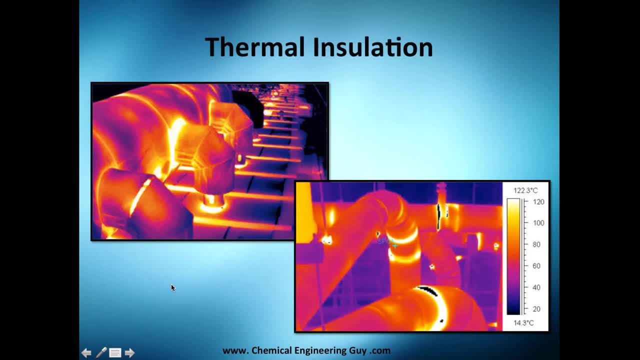 You got small pumps And, yeah, That's the micro reactor trend. Now, just to let you know about thermal insulation. You've seen this in heat energy Or mass balance, Maybe heat transport operations, Whatever, But I'm going to explain you once again. 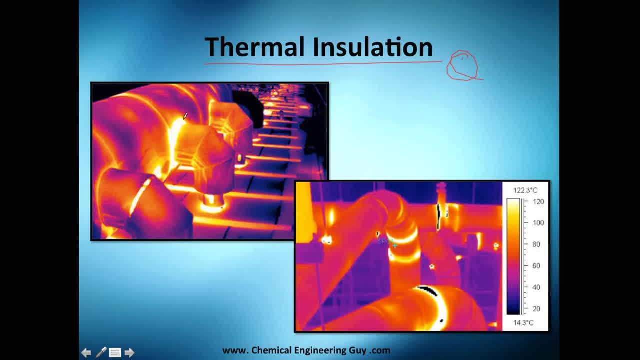 Just to let you know. So these spots right here, This is with the thermal camera, All these, As you can see, If it's yellow It's hot, Or let's say, it's a high temperature, And if it's black, 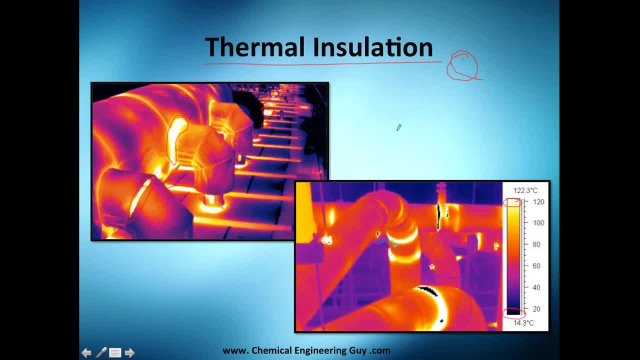 It's low temperature. So what you want to do is low temperatures, Because the ambient temperature will be around 25 Celsius Or 75. It's about like that. So You don't want high temperature, Because high temperatures implies there's a difference in temperature. 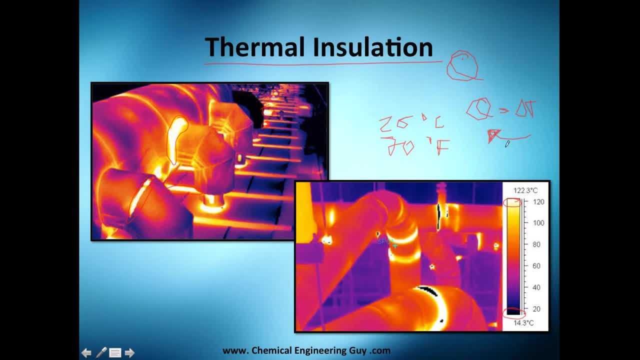 And difference in temperature means that you're going to lose heat With the ambient temperature Or the ambient air. So you don't want that. You want to avoid all these little points here. And how do you do that? You do it by isolating. 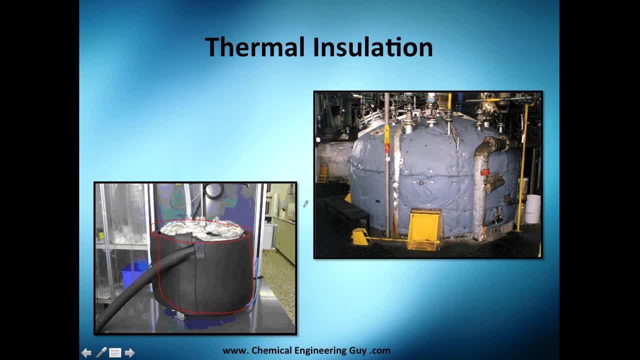 Or thermally isolating the reactor. So look at this: Instead of losing all the heat, You just cover the reactor, Cover the inlets Or all the piping, And you get this kind of arrangement. So look at this, You have all these pipes are covered. 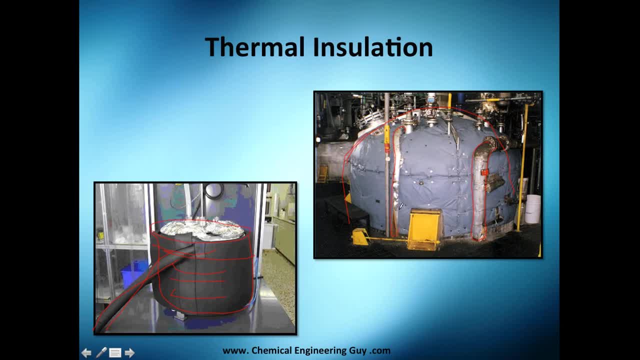 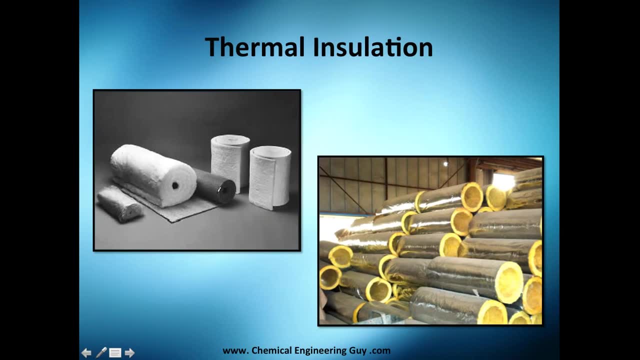 This is not metal. This is isolating material And you also cover the heating vessel. What type of material you use? They use a lot, But this is how they look. It's like a foam like, Or like asbestos like. You also use liquid. 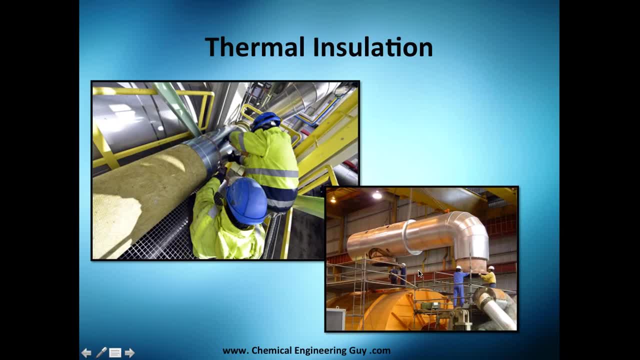 You cover it with aluminium. And yeah, Essentially that's the thermal isolation. One thing I want you to let you know is: Let me go to the next picture. I remember going to my first chemical industry And I thought these were pipes. 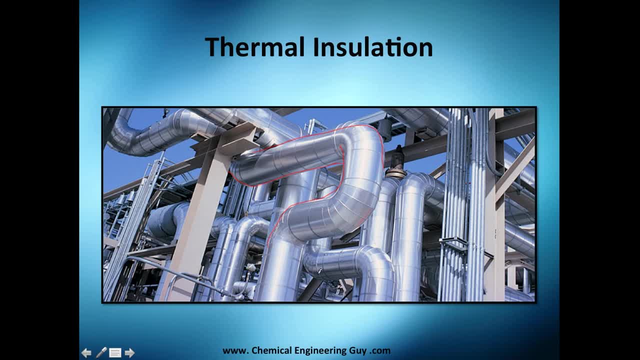 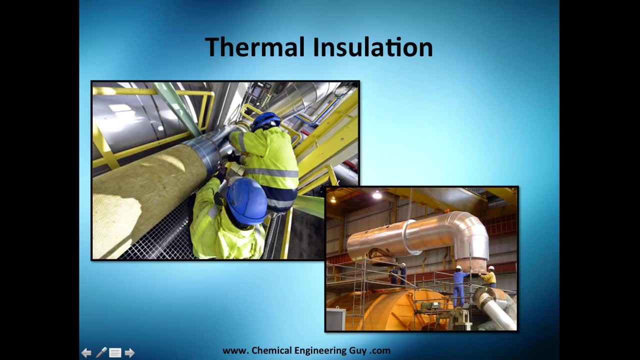 And I wasn't that bad Because there are actually pipes inside of it, But I thought these were the whole pipes And that's not true. actually, You got this isolation inside this, Inside this metal, So you see the pipe here. It's actually covering the isolation material. 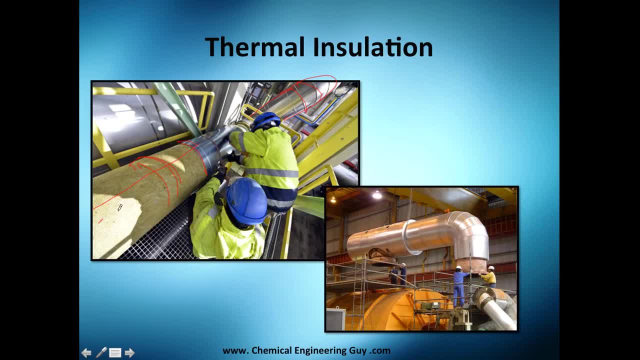 So maybe the actual size of this pipe will be. I don't know This size. So, even though you see a huge pipe Or a huge tube here, You got this small tube here Because it's super hot And you got around it all this material. 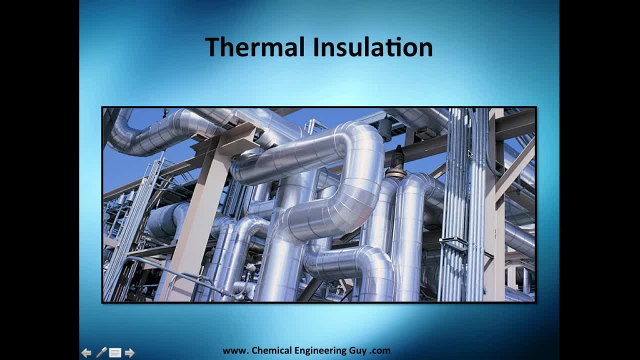 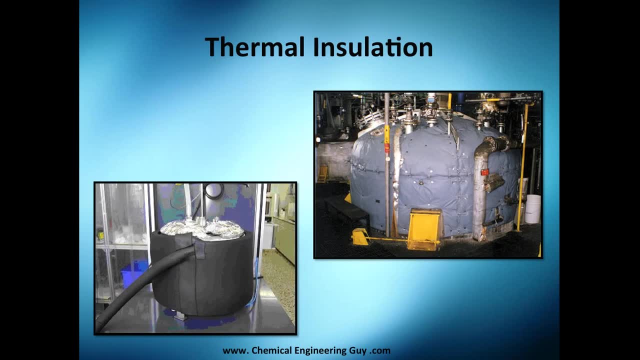 So that's about thermal isolation. Just an overview So you can Know Like There's Isolating Problems in reactors. So if you want to keep a temperature, For example, you want to be At the same temperature as a thermal 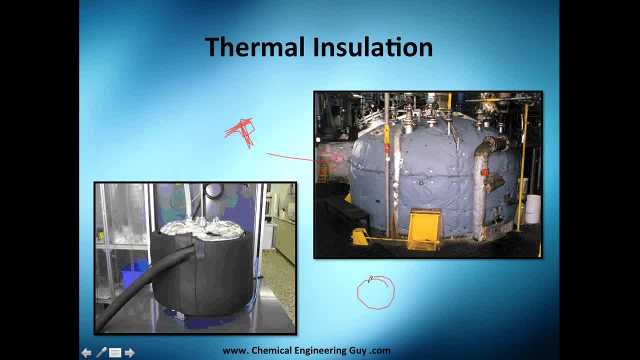 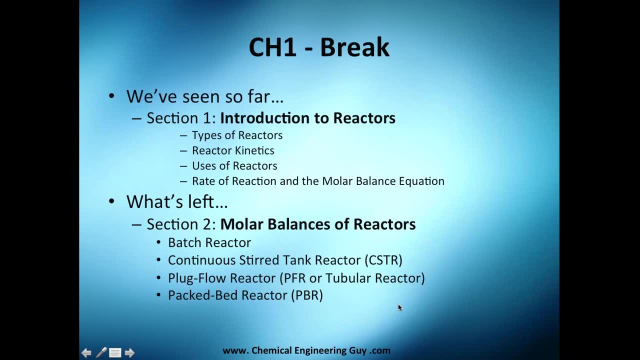 You will need to take care about that. Or if simply you don't want to spend that much money In heat requirement, You will need to buy some isolation material, And that's everything for this section. Section number one: Let me tell you what. 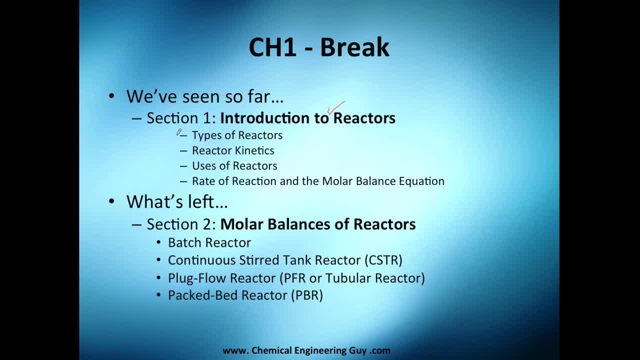 We've seen so far. We saw a small interaction to reactors, Type of reactors, Reactor kinetics, The uses of these reactors, And well, This is I just move it to here. What's left is section two: Molar balances of batch reactor. 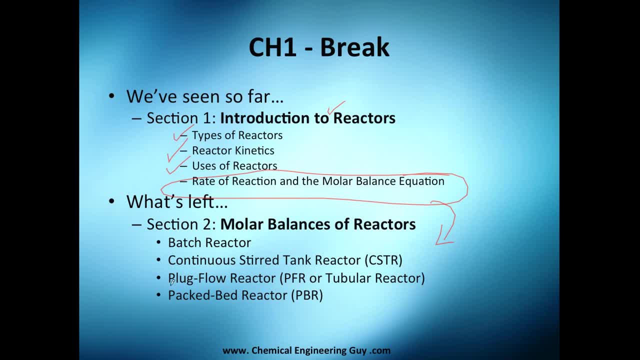 Continuous Steer tank reactors, Plug flow reactors, Pack bed reactors. We're going to see Now the mathematics And we're going to derive an equation That help us to Model these Four Reactors. So thank you for watching, guys. 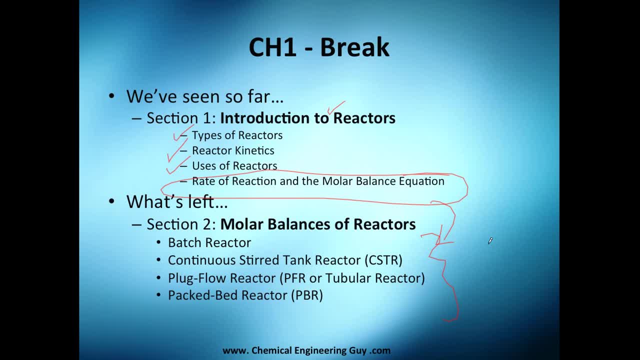 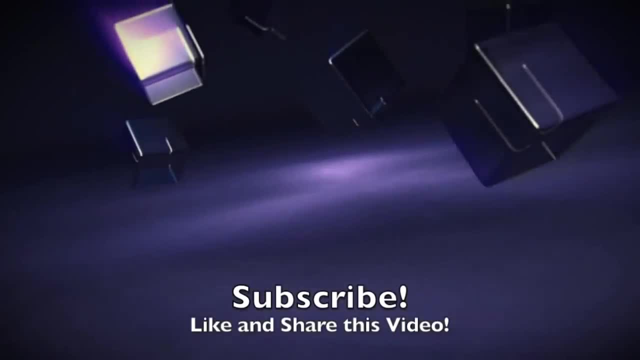 If you are interested In how We can model these tanks Or these reactors, Please Just go to the next video. What's up guys? It's me Chemical engineering guy. So if you like the video, Why not Push the like button? 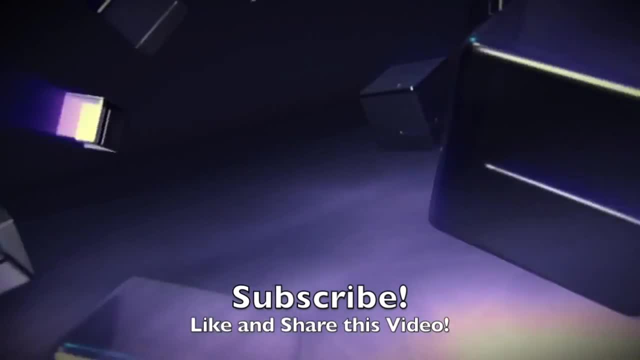 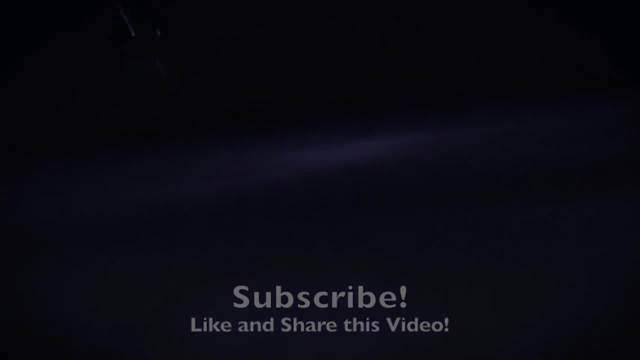 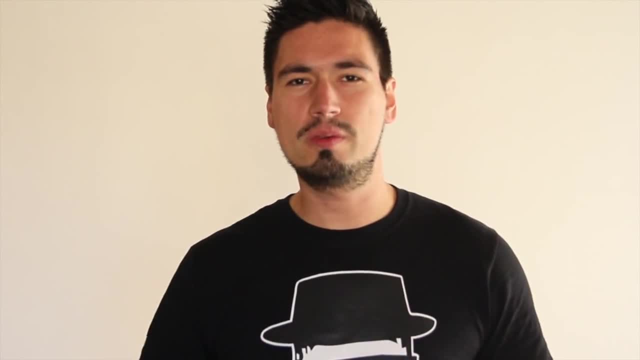 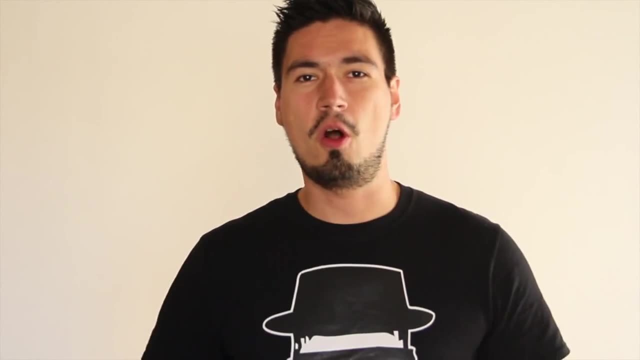 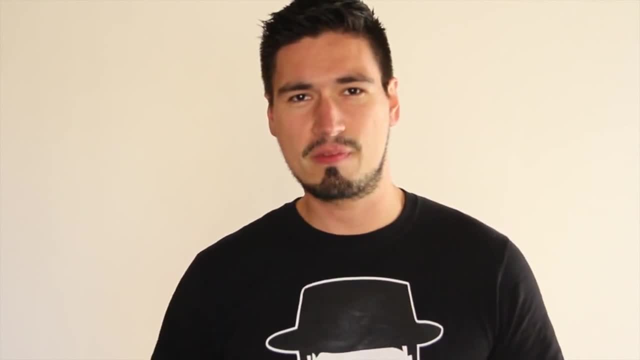 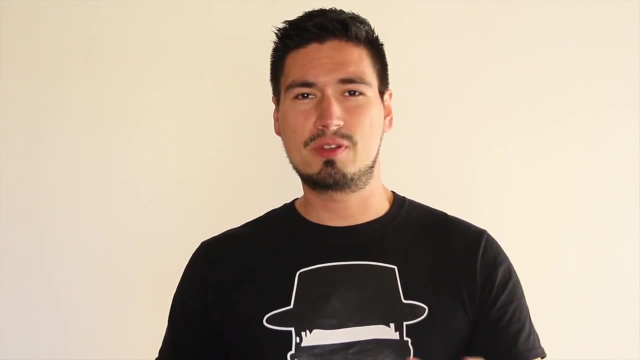